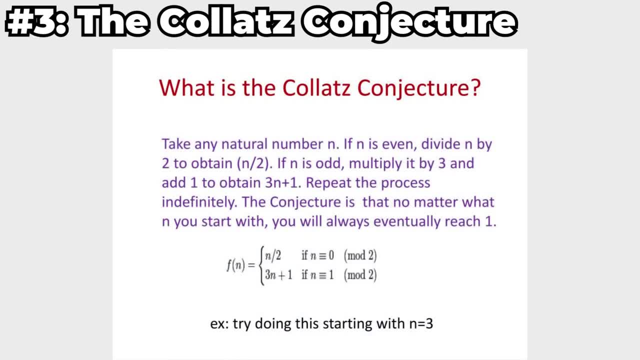 but no one has been able to provide a conclusive proof. Number 3. The Collatz Conjecture. The Collatz Conjecture deals with a simple iterative algorithm applied to positive integers. The algorithm states that if the number is even divided by 2,, 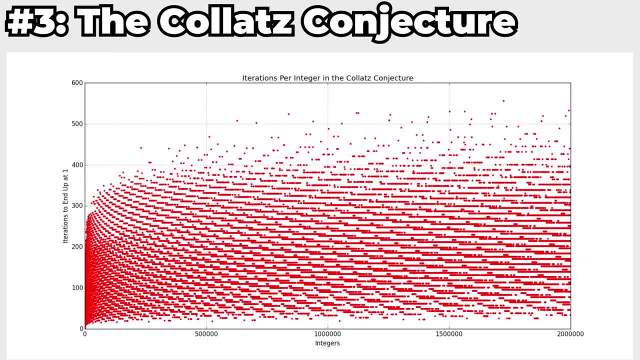 add odd, multiply it by 3, and add 1.. The conjecture proposes that no matter what positive integer you start with, the sequence will eventually reach the number 1.. While this seems to hold true for all numbers tested so far, no one has been able to provide a rigorous proof. 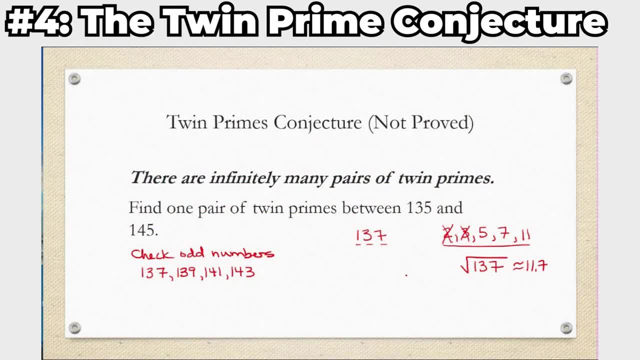 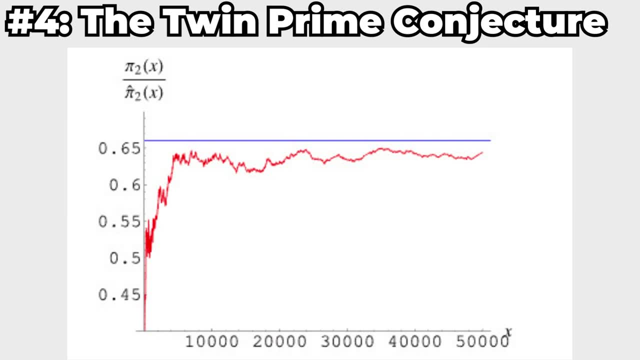 Number 4. The Twin Prime Conjecture. The Twin Prime Conjecture states that there are infinitely many pairs of primes that differ by 2, eg 3 and 5,, 5 and 7,, etc. While there are many examples of such pairs, 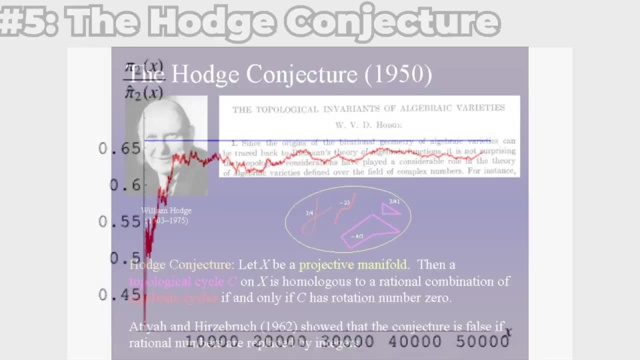 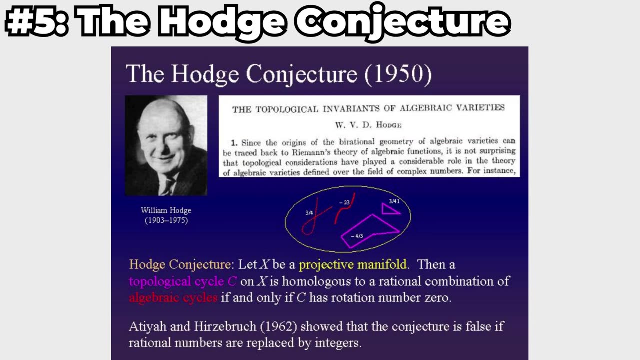 no one has been able to prove that there are infinitely many Number 5.. The Hodge Conjecture. The Hodge Conjecture deals with the relationship between algebraic and topological properties of certain geometric objects. Specifically, it proposes that certain cohomology classes can: 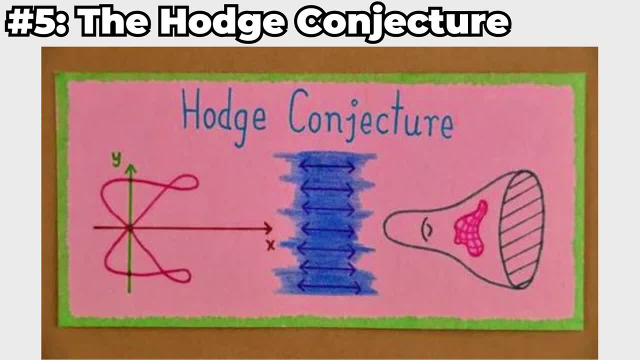 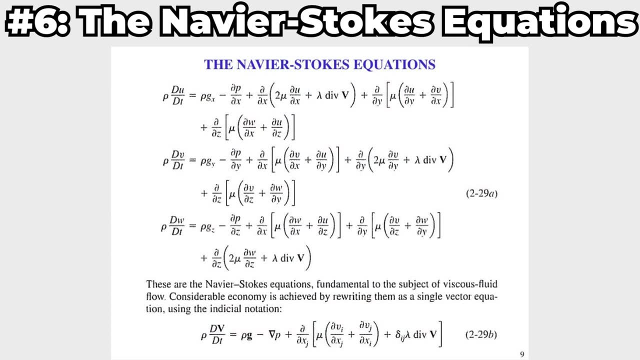 be represented by algebraic cycles. While the conjecture has been verified in some cases, a general proof remains elusive. Number 6. The Navier-Stokes Equations. The Navier-Stokes Equations describe the motion of fluids and are used in fields such as aerodynamics and oceanography. 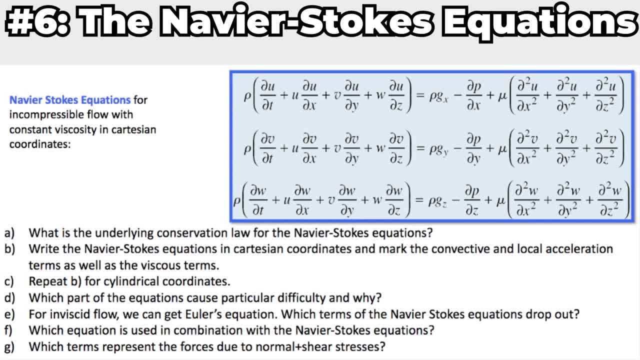 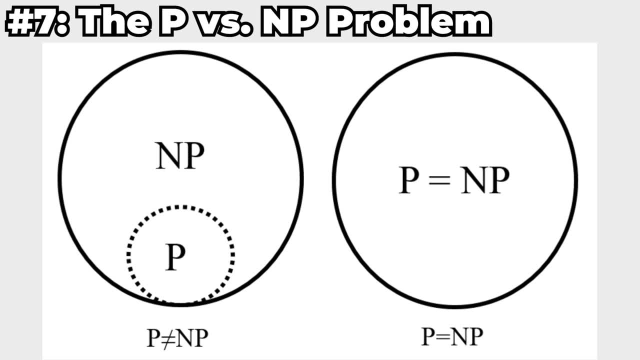 While they have been around for over 150 years, a general proof of their existence and uniqueness of solutions remains elusive. Number 7. The P vs NP Problem. The P vs NP problem deals with the complexity of computational problems. Specifically, it asks whether problems that can be solved in polynomial time. 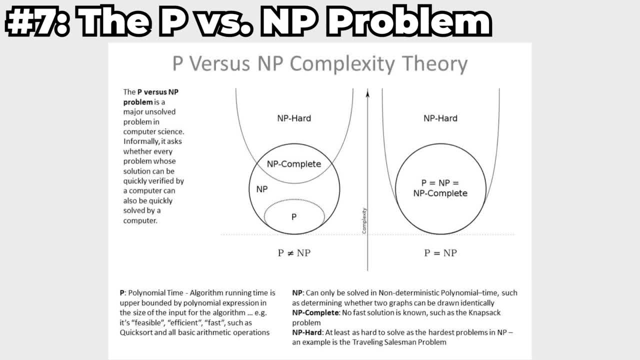 by a non-deterministic computer can also be solved in polynomial time by a deterministic computer. While it is widely believed that P is not solvable in polynomial time, no one has been able to provide a proof. Number 8. The Birch and Swinerton-Dyer Conjecture. 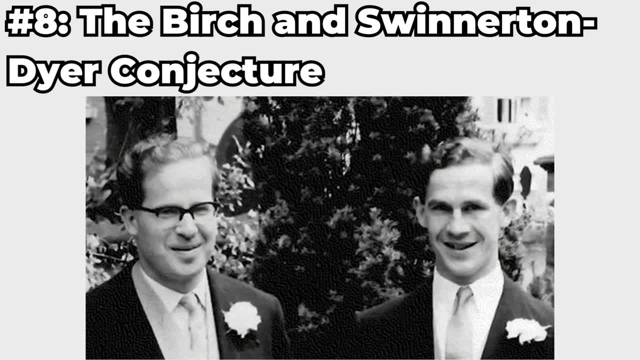 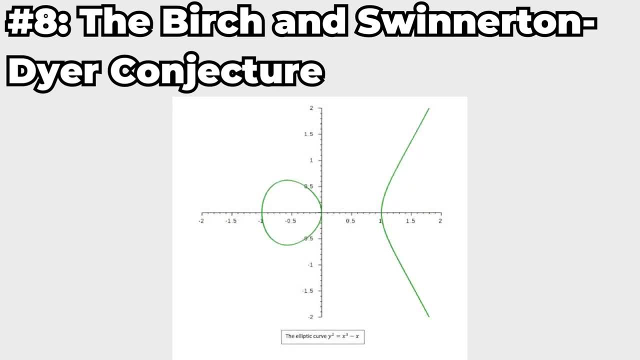 The Birch and Swinerton-Dyer Conjecture deals with elliptic curves, which are important objects in number theory. The conjecture proposes a relationship between the number of points on an elliptic curve and certain algebraic properties of the curve. While the conjecture has been verified in some cases, a general proof remains elusive.